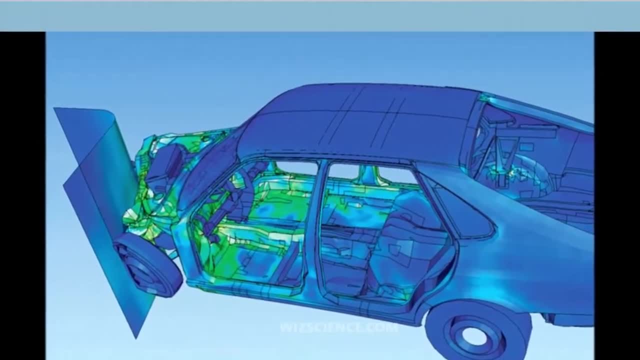 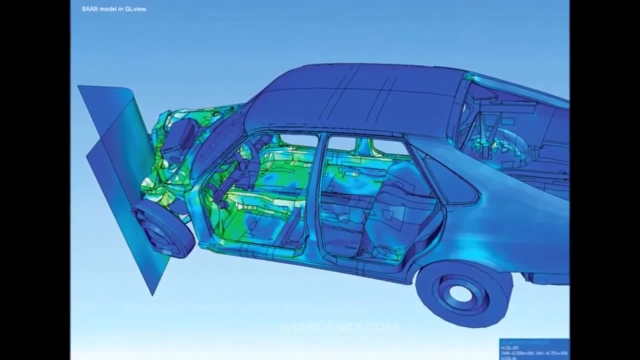 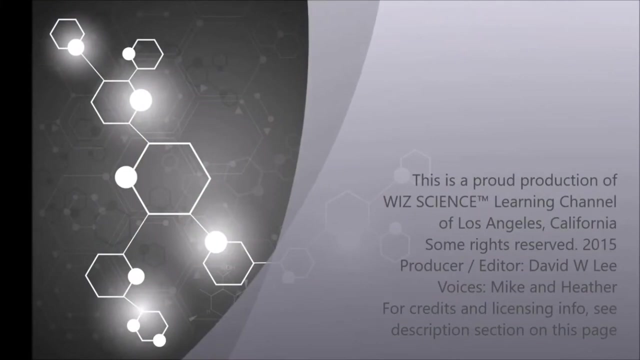 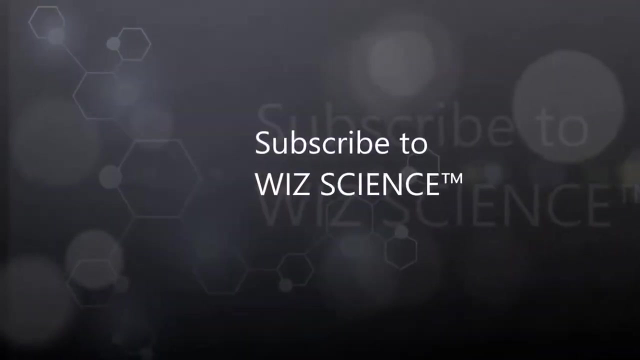 where they will more than likely assist in building treatment facilities, preparing environmental impact assessments or helping to mitigate air pollution from specific point sources. Thank you for watching. For more educational information, please visit our website at wwwunedu For more educational videos. please subscribe to WhizScience on YouTube or visit whizsciencecom. 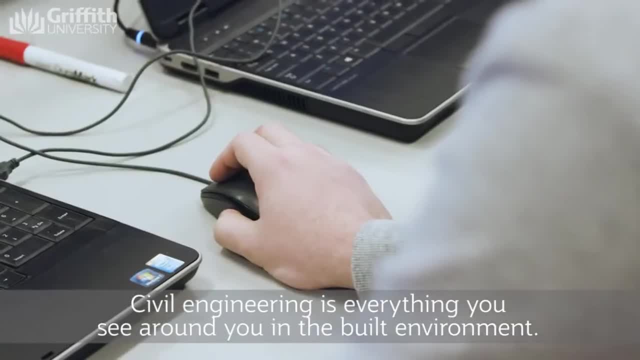 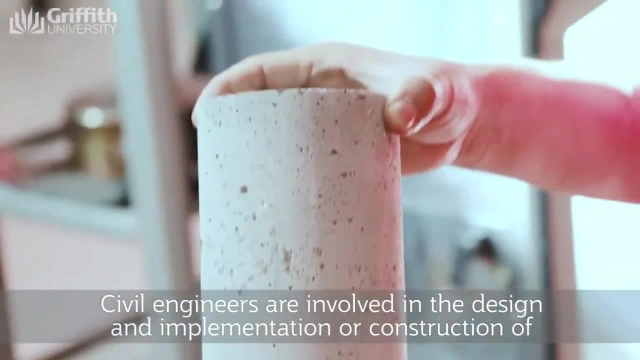 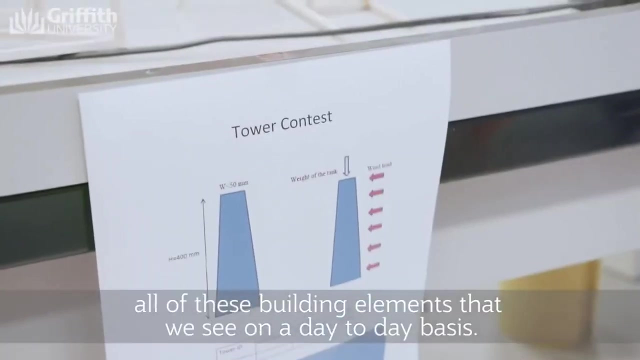 Civil engineering is everything that you see around you in the built environment, the roads that you drive on. it's the buildings that you go into. Civil engineers are involved in the design and implementation or construction of all of these building elements that we see on a day-to-day basis. In our new Bachelor of Engineering with honors, the students can: 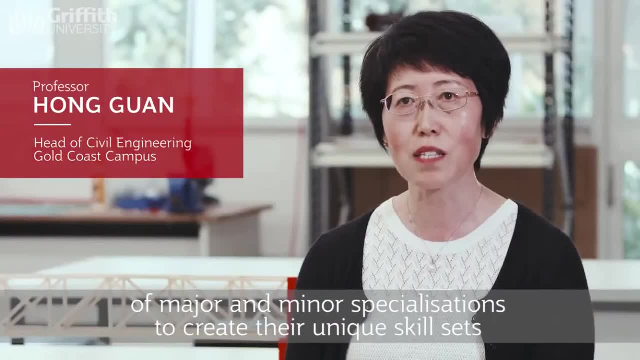 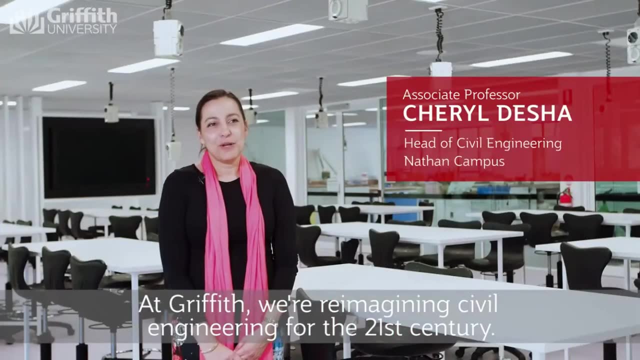 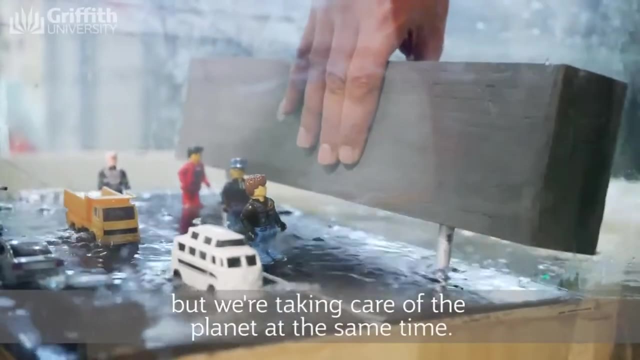 choose from a wide range of majors and minor specializations to create their unique skill sets and also gain knowledge for their dream job. At Griffith, we're reimagining civil engineering for the 21st century. We need to make sure that we're not only taking care of human beings, but we're taking care of the planet. at the 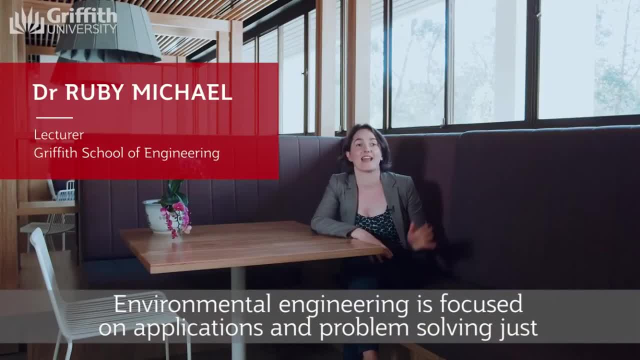 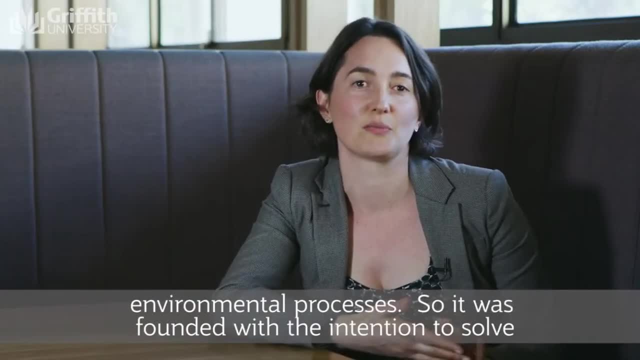 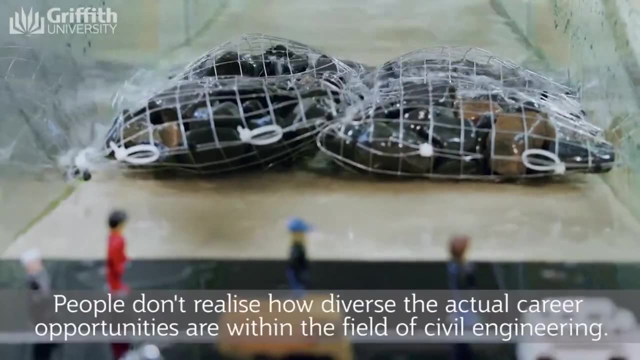 same time, Environmental engineering is focused on applications and problem solving, just like every other engineering discipline, But environmental engineering is underpinned by environmental processes, So it was founded with the intention to solve some of our biggest problems globally. People don't realize how diverse the actual career opportunities are within the field. 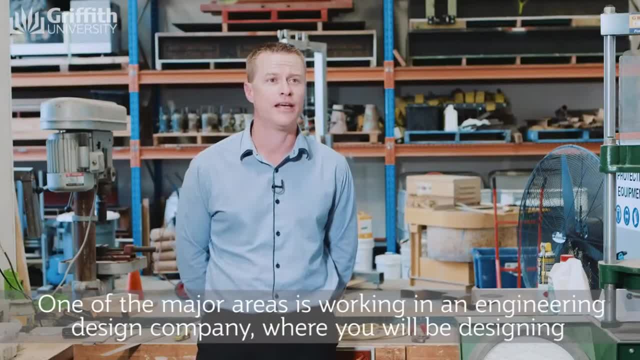 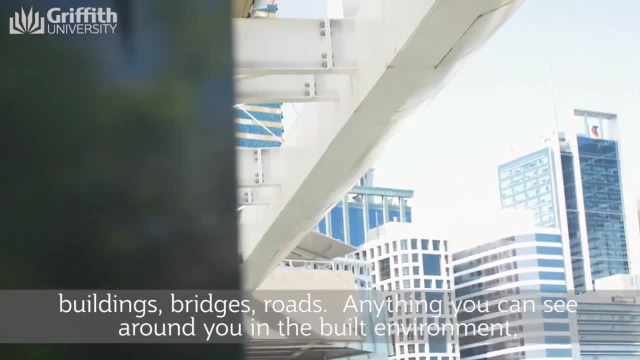 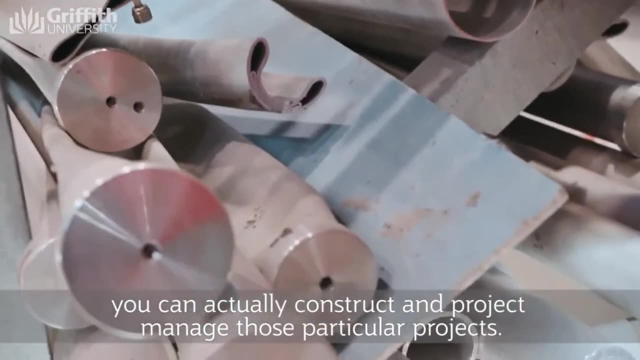 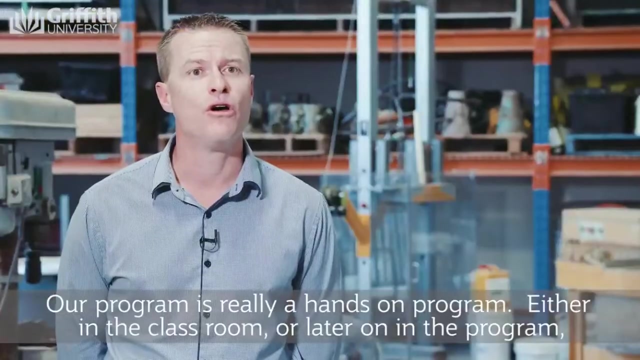 of civil engineering. One of the major areas is working in an engineering design company where you will be designing buildings, bridges, roads- anything that you see around you in the built environment. you can actually construct and project manage. Our program is really a hands-on program, either in the classroom or later on in the 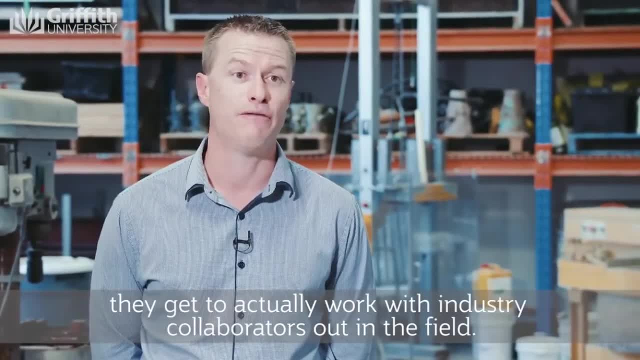 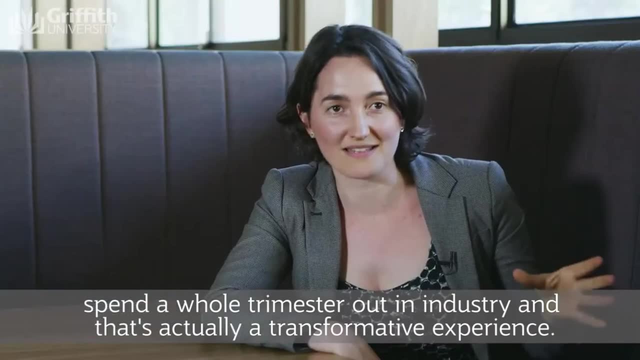 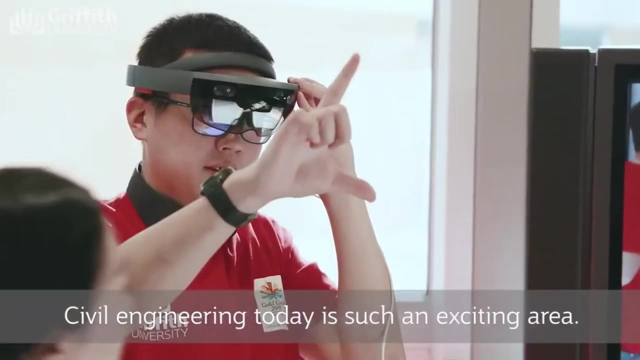 program they get to actually work with industry collaborators out in the field. We have a special program called the Industry Affiliates Program, which actually students spend a whole trimester out in industry and that's actually a transformative experience. Civil engineering today is such an exciting area With seven and a half billion people. living on this planet and attempting to make a difference in the lives of millions of people. it's a really exciting experience. Civil engineering today is such an exciting area, with seven and a half billion people living on this planet and attempting to make a difference in the lives of millions of people. 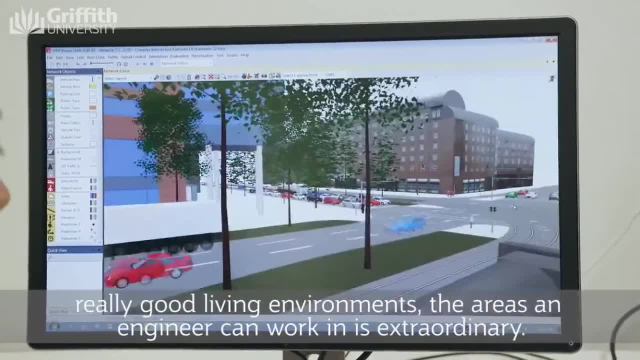 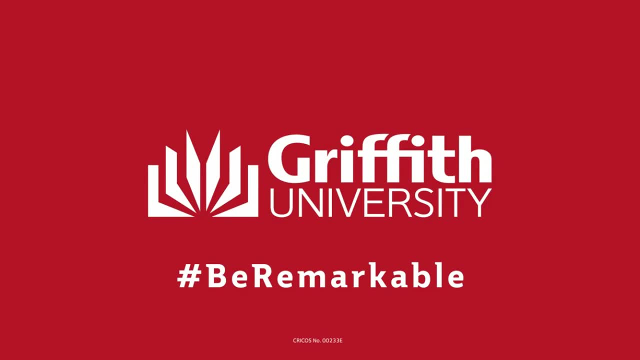 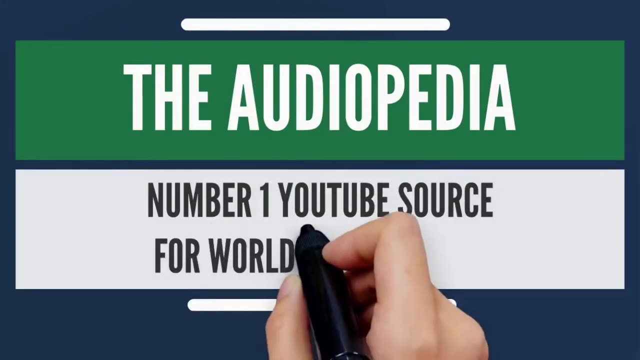 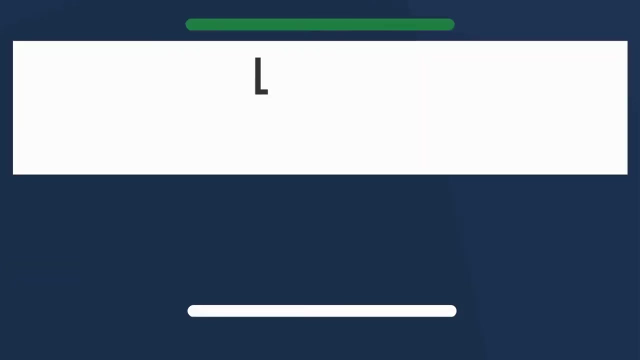 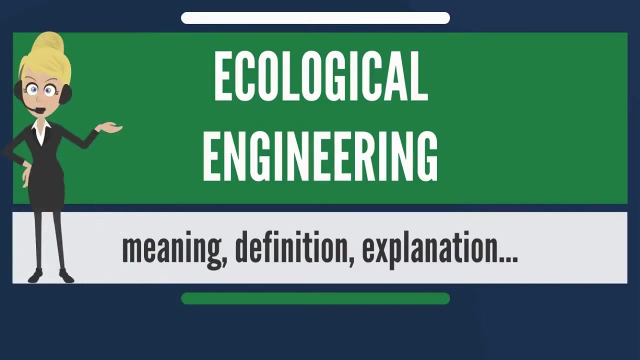 to access really good transportation, really good living environments. The areas that a civil engineer can work in is extraordinary. The areas that a civil engineer can work in is extraordinary. Ecological engineering is an emerging study of integrating ecology and engineering concerned with the design, monitoring and construction of ecosystems. 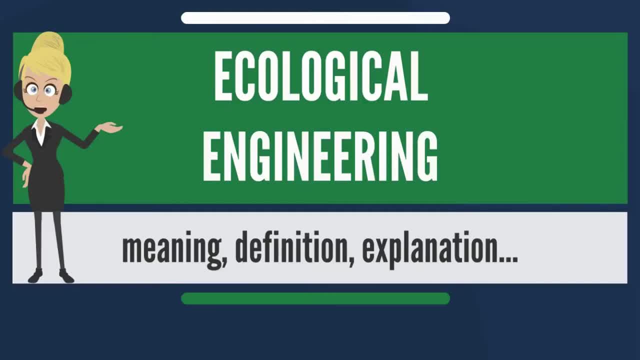 The design of sustainable ecosystems intends to integrate human society with its natural environment for the benefit of both. Ecological engineering emerged as a new idea in the early 1960s, but its definition has taken several decades to refine. its implementation is still undergoing adjustment, and its broader 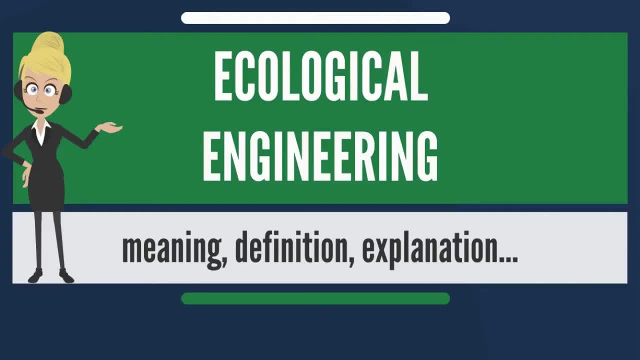 recognition as a new paradigm is relatively recent. Ecological engineering was introduced by Howard Odom in the 1960s- Odom and others as utilizing natural energy sources as the predominant input to manipulate and control environmental systems. Mitch and Jorgensen wrote that ecological engineering is designing societal services. 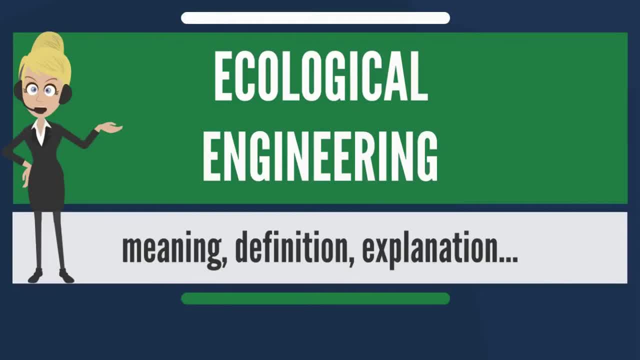 such that they benefit society and nature, and later noted the design should be systems-based, sustainable and integrate society with its natural environment. Odom emphasized that self-organizational properties were a central feature to ecological engineering and that it was a fundamental part of the development of ecological engineering. 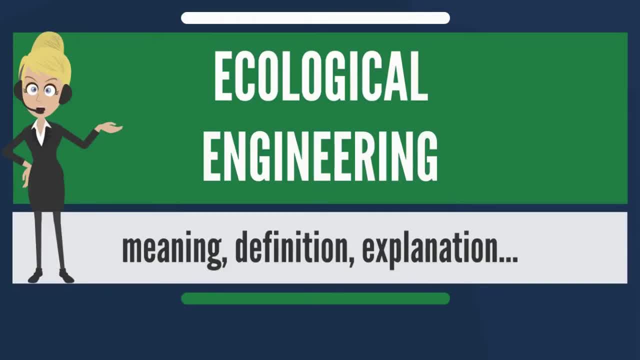 Mitch and Jorgensen were the first to define ecological engineering and provide ecological engineering principles. Later they refined the definition and increased the number of principles. They defined and characterized ecological engineering in a 1989 book and clarified it further in their 2004 book, Sea Literature. 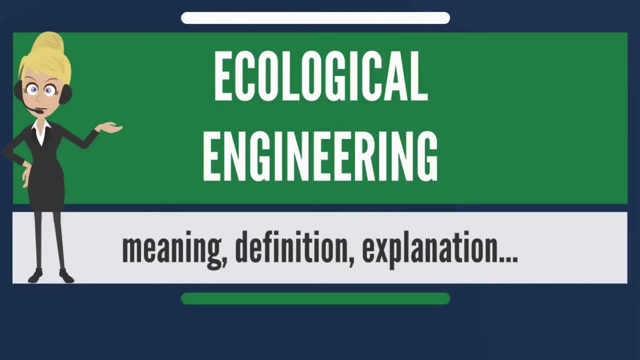 They suggest the goal of ecological engineering is the restoration of ecosystems that have been substantially disturbed by human and animal activities, such as environmental pollution or land disturbance, and the development of new sustainable ecosystems that have both human and ecological values. They summarized the five concepts key to ecological engineering as: 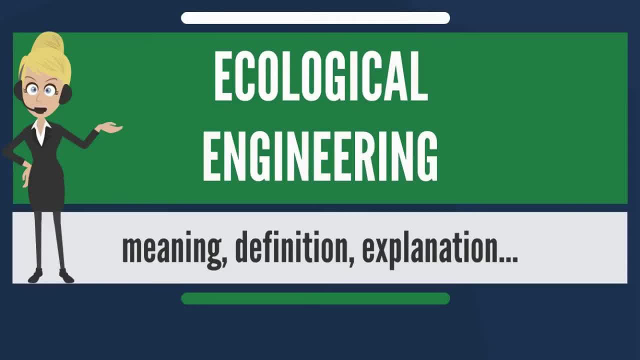 1. It is based on the self-designing capacity of ecosystems. 2. It can be a field test of ecological theory. 3. It relies on integrated system approaches. 4. It conserves non-renewable energy and 5.. 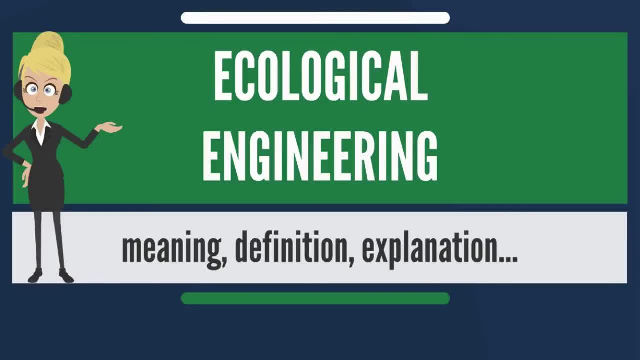 It supports biological conservation. Bergen et al defined ecological engineering as: 1. Utilizing ecological science and theory, 2. Applying to all types of ecosystems, 3. Adapting engineering design methods and 4. Acknowledging a guiding value system. 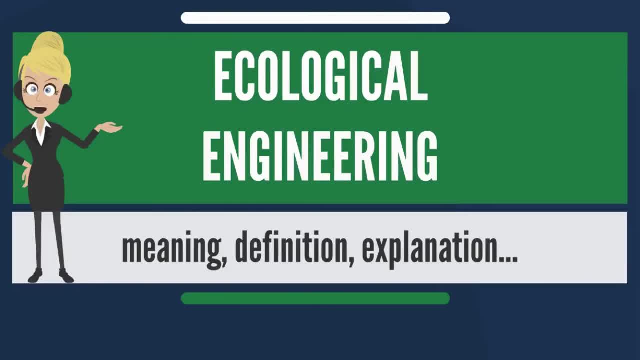 Barrett offers a more literal definition of the term: the design, construction, operation and management- that is engineering- of landscape-slash-aquatic structures and associated plant and animal communities, that is, ecosystems to benefit humanity and often nature. Barrett continues. other terms with equivalent or similar meanings include ecotechnology. 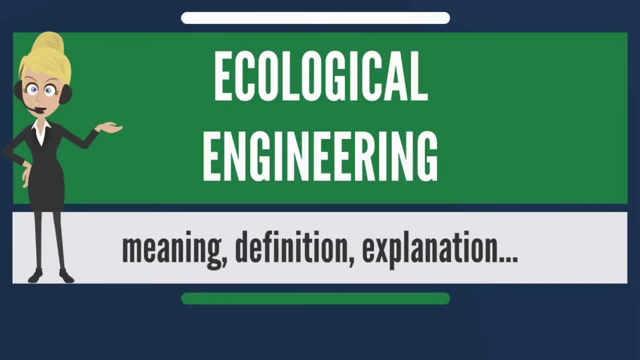 and two terms most often used in the erosion control field soil: bioengineering and biotechnical engineering. However, ecoengineering should not be confused with biotechnology when describing genetic engineering at the cellular level, or bioengineering meaning construction of artificial body parts. 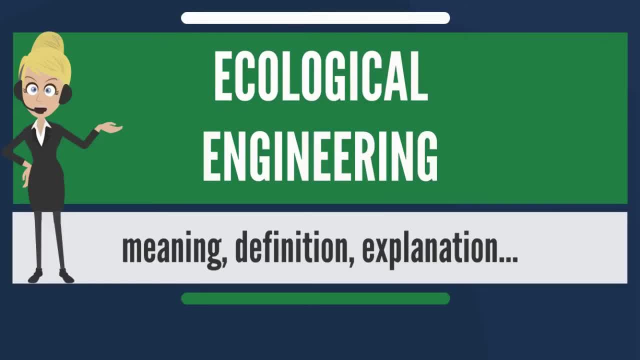 This engineering discipline combines basic and applied science from engineering, ecology, economics and natural sciences for the restoration and construction of aquatic and terrestrial ecosystems. The field of ecological engineering is in the field of ecological engineering. The field of ecological engineering is in the field of environmental engineering, and. 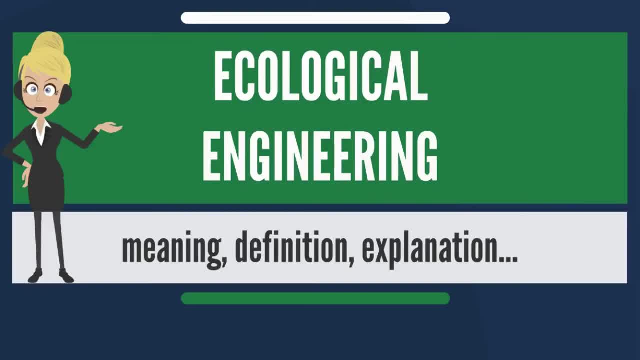 is increasing in breadth and depth as more opportunities to design and use ecosystems as interfaces between technology and environment are explored. Implementation of ecological engineering has focused on the creation or restoration of ecosystems from degraded wetlands to multi-celled tubs and greenhouses that integrate microbial, fish and plant services to 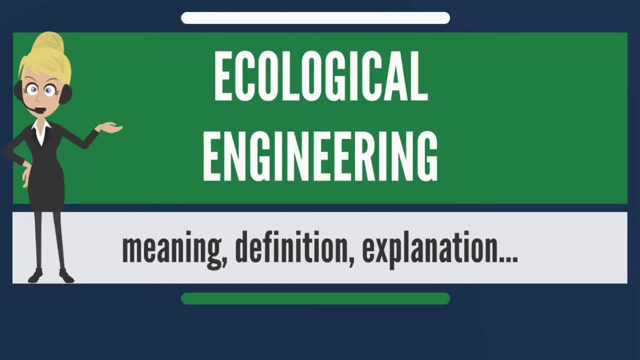 process human wastewater into products such as fertilizers, flowers and drinking water. Potential applications of ecological engineering in cities have included the field of landscape architecture, urban planning and urban horticulture, which can be synthesized into urban stormwater management. Potential applications of ecological engineering in rural landscapes have 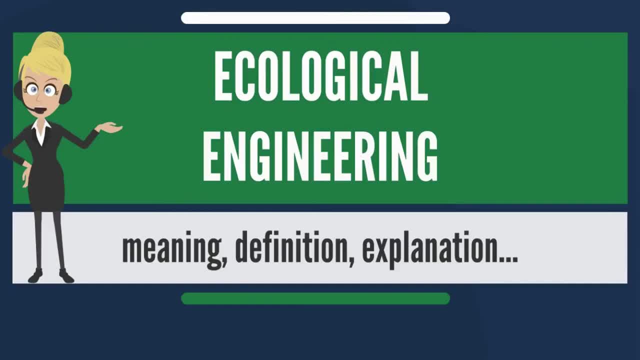 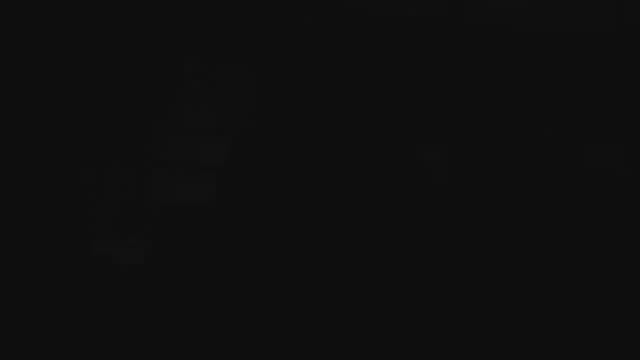 included wetland treatment and community reforestation through traditional ecological knowledge. Recent lifestyle and habitat planning examples include the permaculture movement. Potential applications of ecological engineering include the permaculture movement. Potential applications of ecological engineering include the permaculture movement. 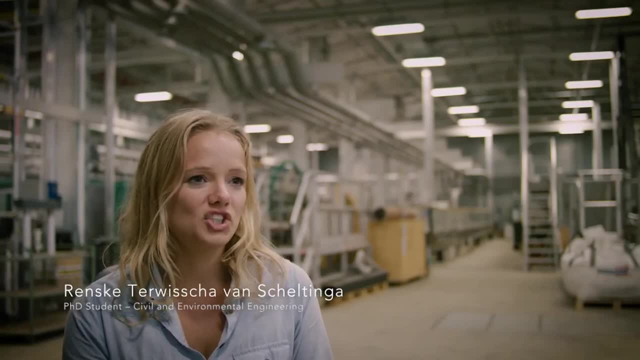 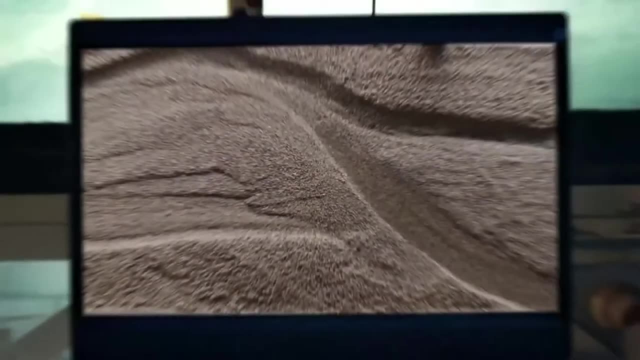 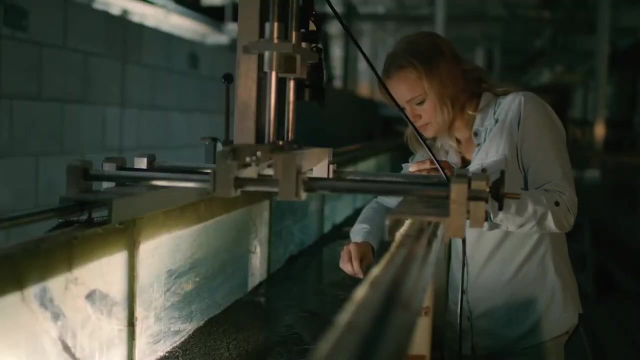 My name is Renske Terwischa van Scheltinga. I am a PhD student. I was born in the Netherlands. We are in the hydraulic engineering laboratory of the University of Auckland where we just recorded a video of my flume experiment. This is one of the top places to do research around. 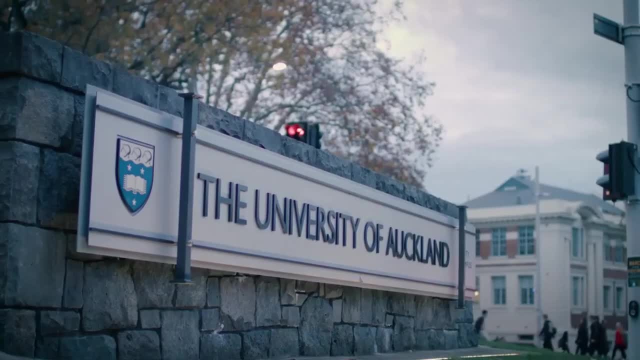 the world because of its facilities and because of the big forest. Potential applications of ecological engineering include the permaculture movement. Potential applications of ecological engineering include the permaculture movement. Potential applications of ecological engineering include the permaculture movement. Potential applications of ecological engineering include the. 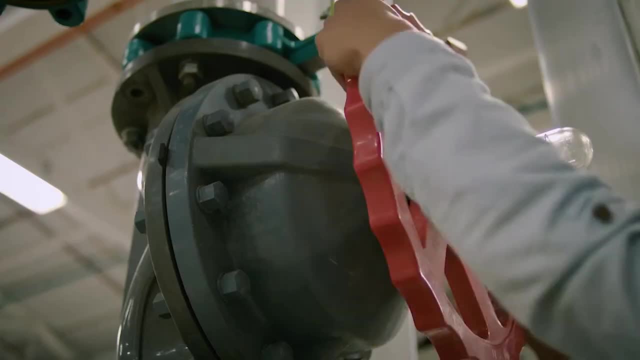 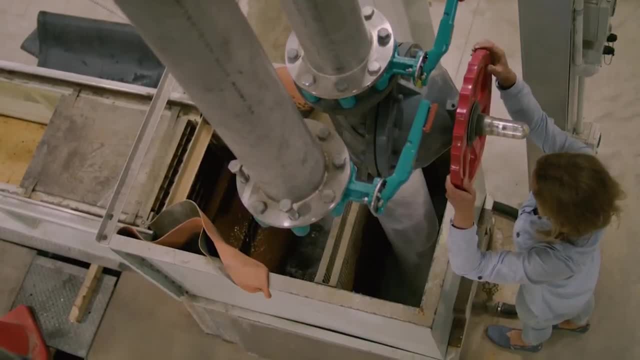 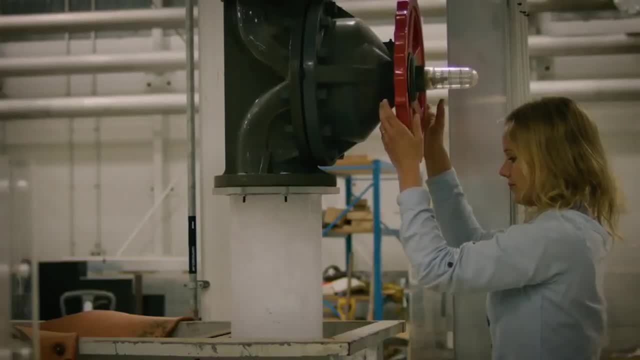 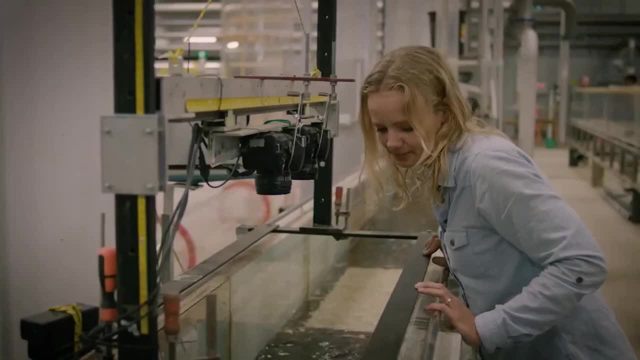 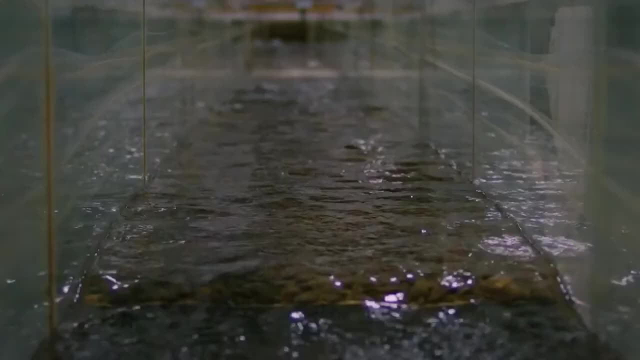 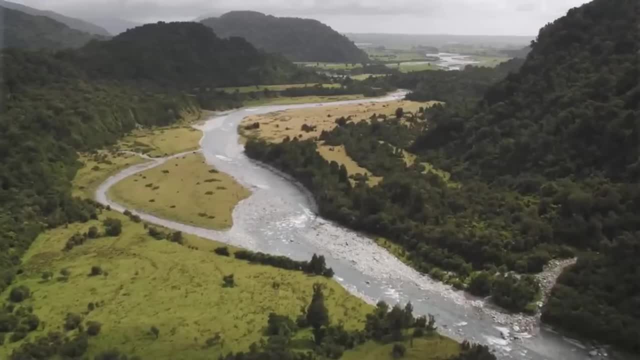 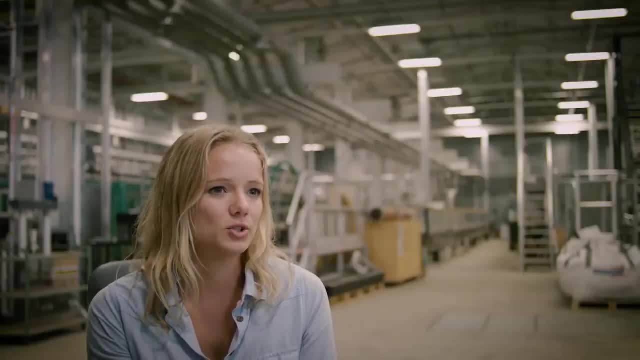 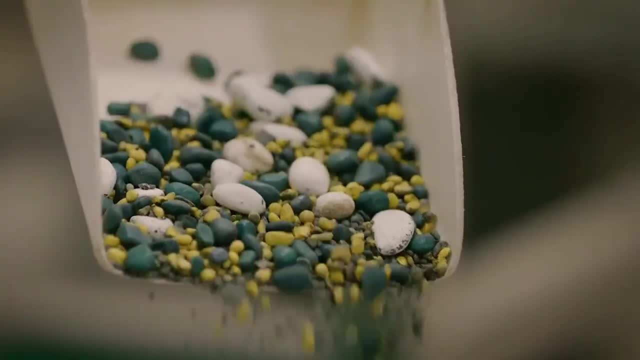 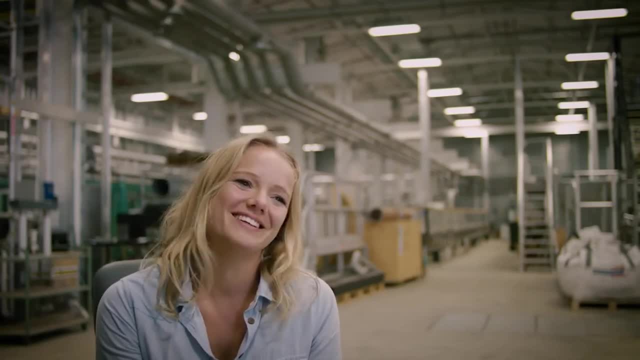 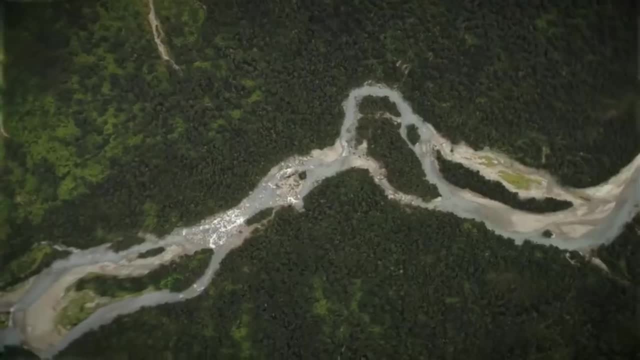 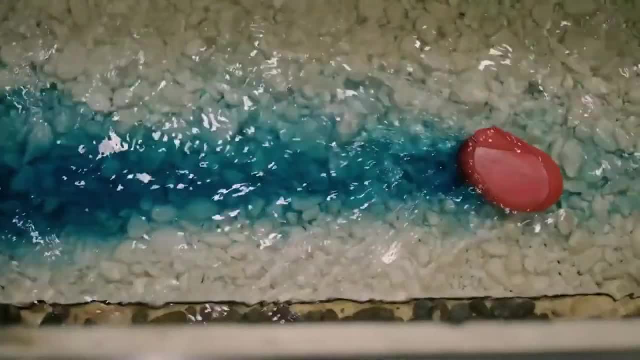